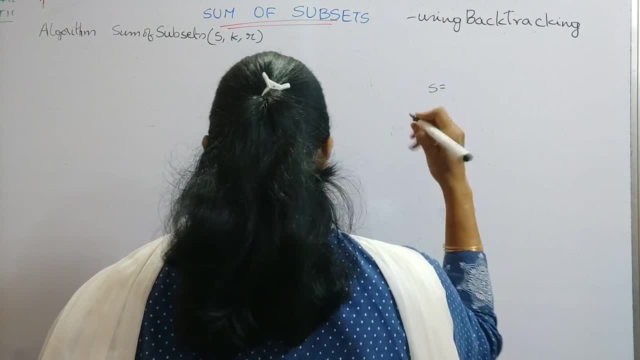 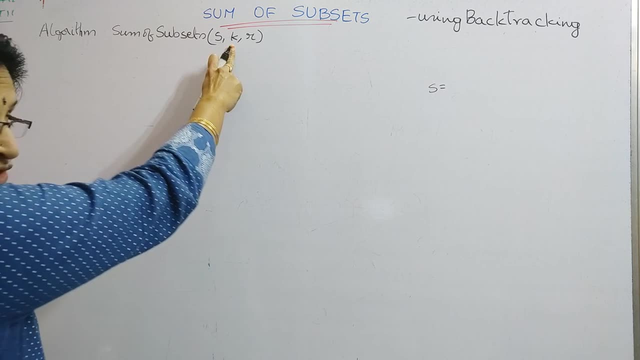 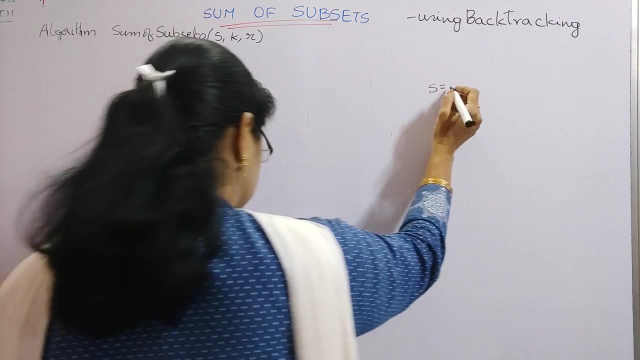 say that S is equal to, it is the decision up to the kth object. So that means: suppose, if you are taking the decision of the kth object whether it should be given or not. So this is, S indicates the previous decision. So that is, it is equal to. k is equal to. 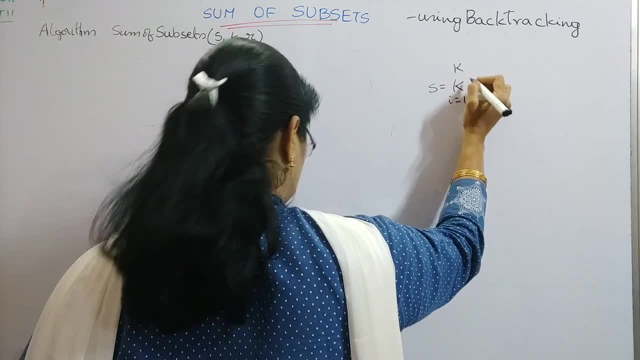 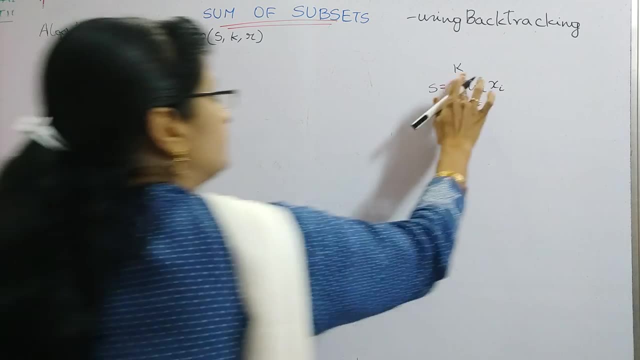 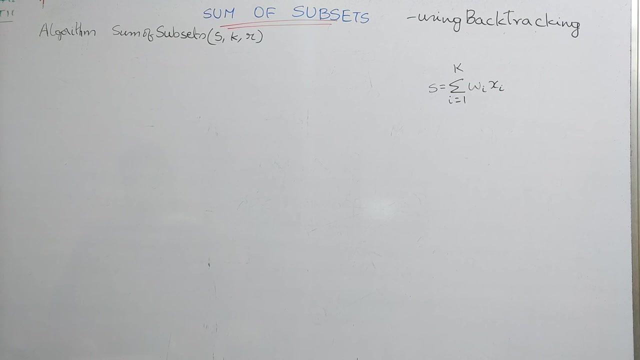 1, i is equal to 1 to k wi xi. So this is: this is: this is yes. S is equal to i is equal to 1 to k wi xi. Suppose if you are taking the decision for the kth object. So 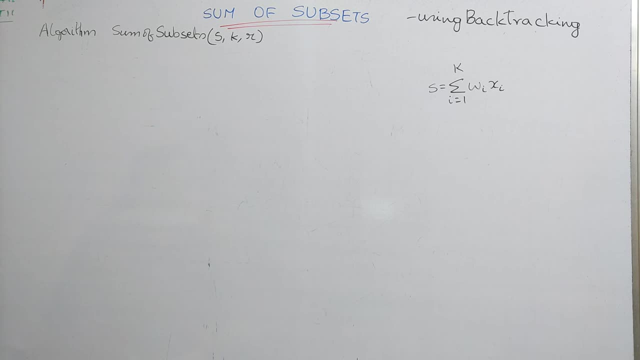 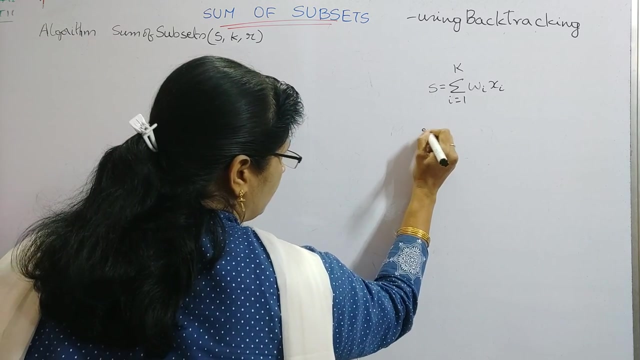 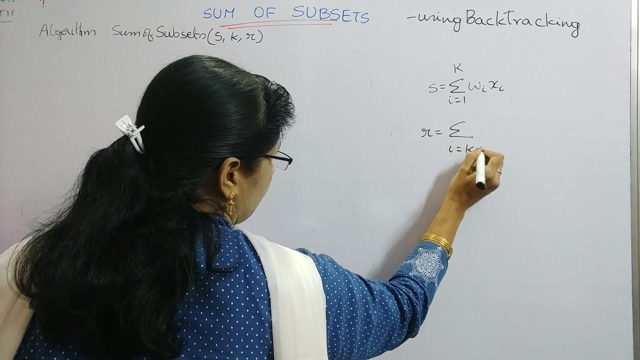 what you are trying to do. You are trying to find the sum of all the objects that are included up to k. And next, what is this R is? R is equal to. it is the sum of the remaining objects, That is, i is equal to. it is from k plus 1 to n. It is from k plus 1 to n and it is the. 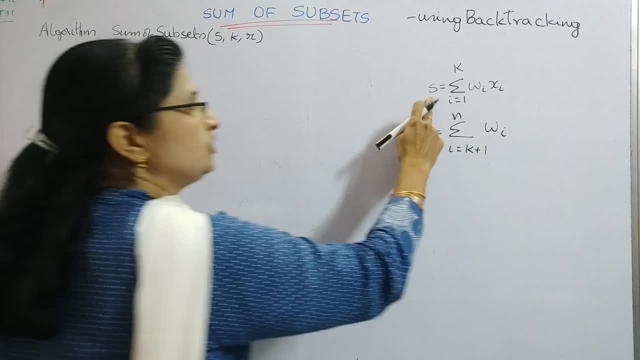 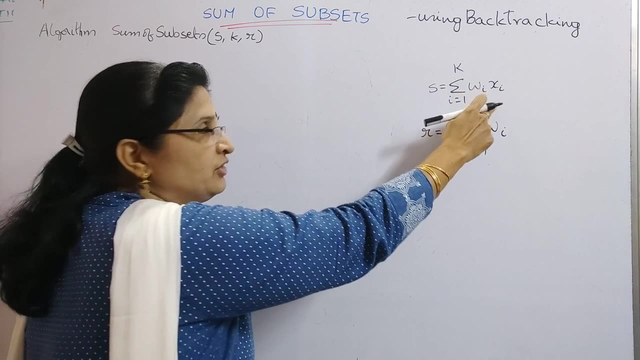 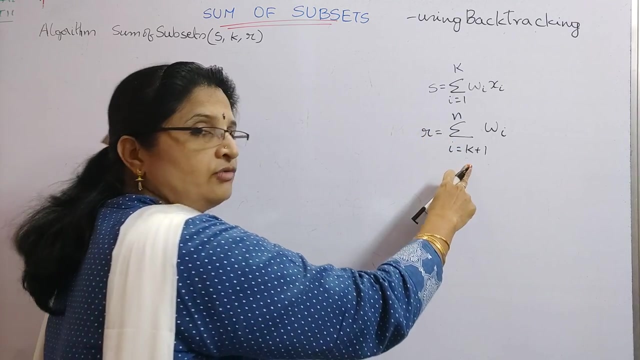 sum of the remaining objects. So here already you have taken the decision up to k objects. So that is why. so whichever objects are added, the sum will be taken for S, But for k plus 1 to n you have not yet taken the decision. So now here what you are doing, You are considering: 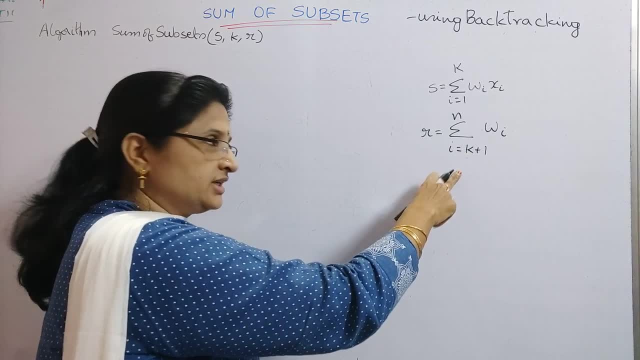 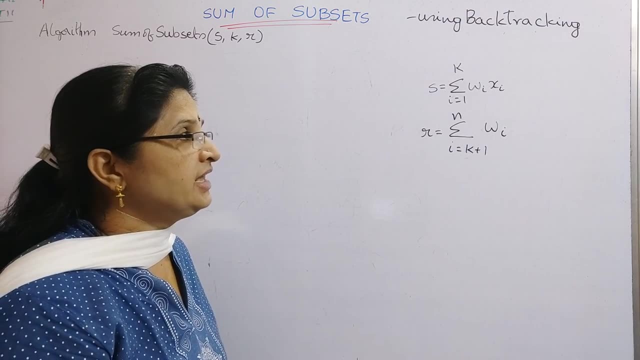 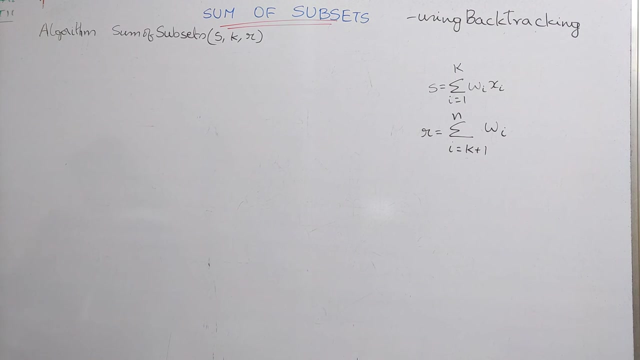 all the objects after the k, So that, because you have not yet considered all these objects, So here we say that the remaining, we say that R is the sum of the remaining objects. So these are the two parameters that you will use for your algorithm and you will use the 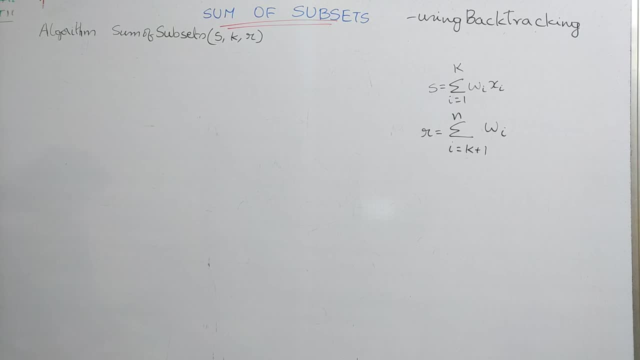 bounding function. So you will use the bounding function. So you will use the bounding function. So you will use the bounding function and you will try to get the solution for your sum of subjects. So first, initially, we will say that x of k is equal to 1. So that means you are giving 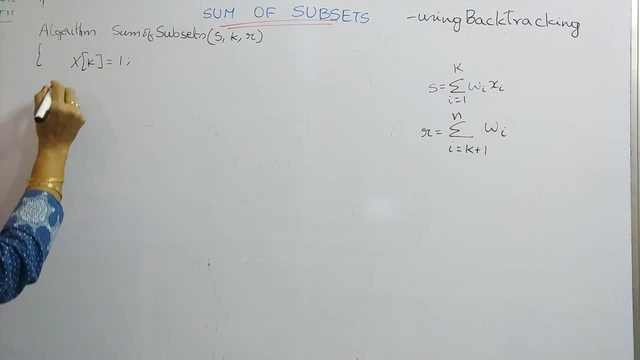 that the kth object is selected. So after giving x of k is equal to 1, so you will check with: yes, That is yes, Yes, OK, Yes, Yes. So the solution is you have to give the solution to the previous decision: w k plus, w k plus. 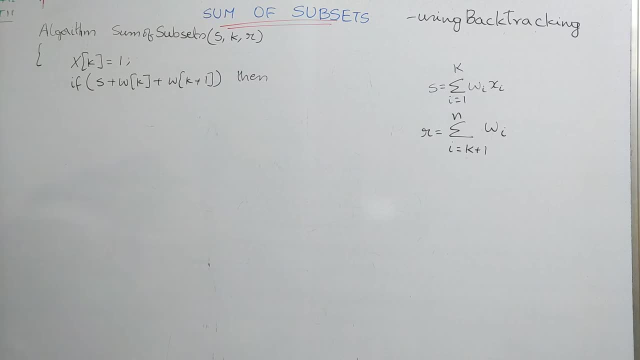 n. So then, sorry, one minute. OK, If s plus w, k plus k, Yes Wk. So that means if Wk, that is, the weight of the kth object, is added to your previous decision. Previous decision is what? 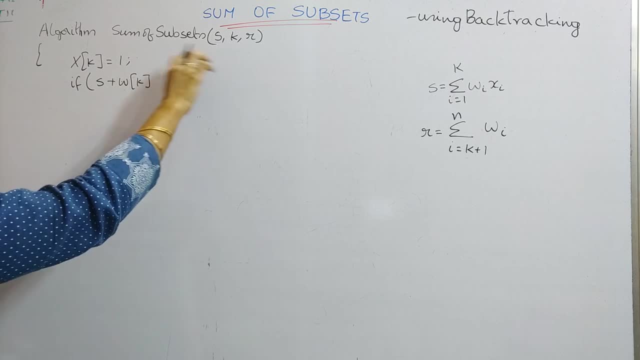 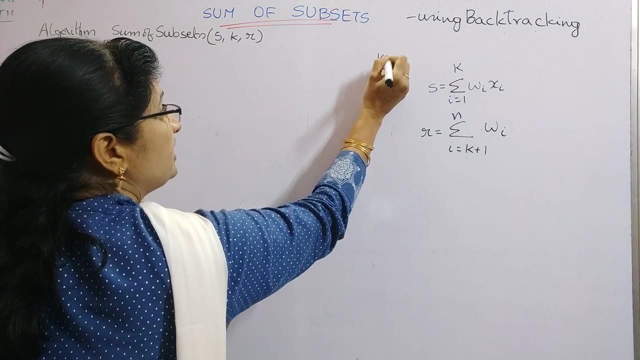 So it will be passed with your function call. So this first, initially, whenever you are accessing this, yes means it indicates that it is the decision up to k minus 1 objects. It is the decision up to k minus 1 objects because this value you will get from. 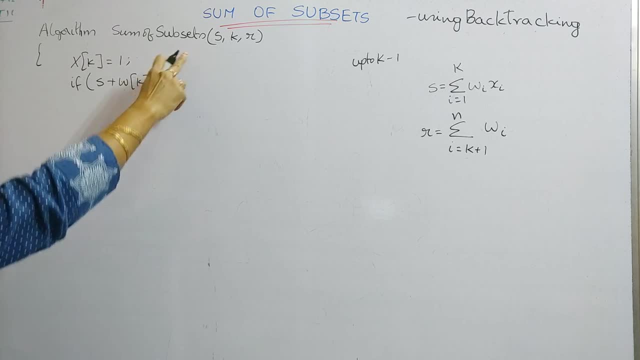 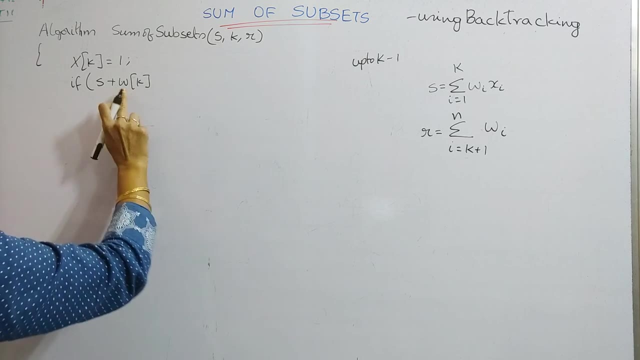 the previous call of your sum of subsets. So that is why it will be the decision up to k minus 1.. So for up you are adding, you are adding the W of k, that is, the weight of the kth. object to the decision. 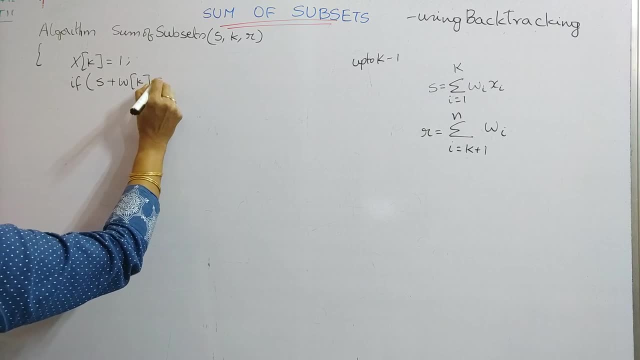 of your k minus 1.. Suppose if this is equal to m. So that means what with k, it has completed. that means, if you are adding the kth object, if it is satisfying your constraint, that is, if it is equal to m. So then what? 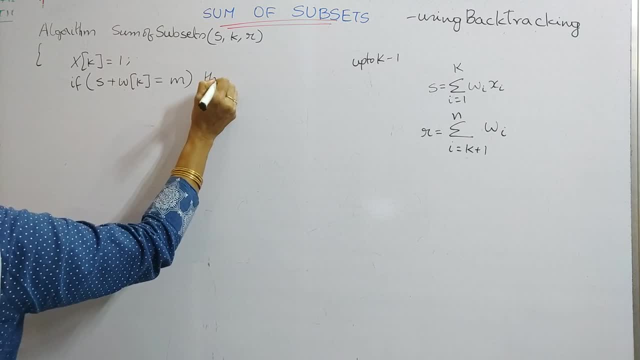 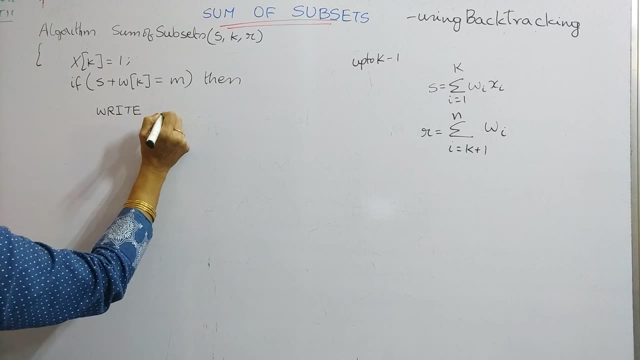 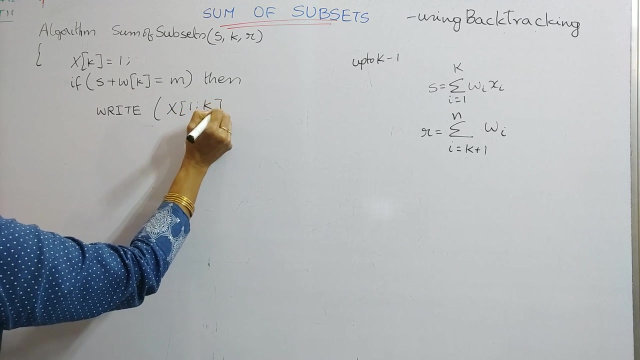 you have to do, You have to write the particular subset. So then, what you have to do, You have to write that particular subset that is from x is equal to 1 to k. So whatever subset you got, so because here the condition is satisfied. 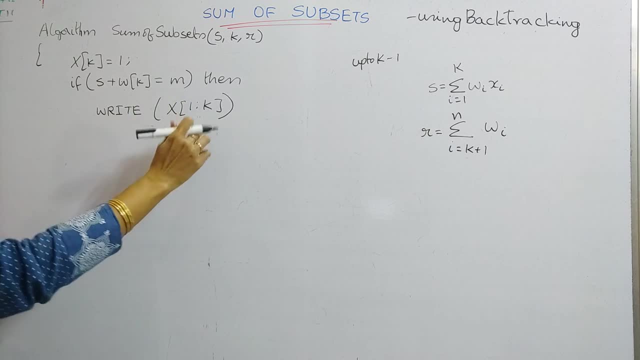 because the sum of subsets is equal to m. So that is why you have to write this particular subset. So suppose, if it is not equal? If it is not equal, So then what you have to do? You have to check. 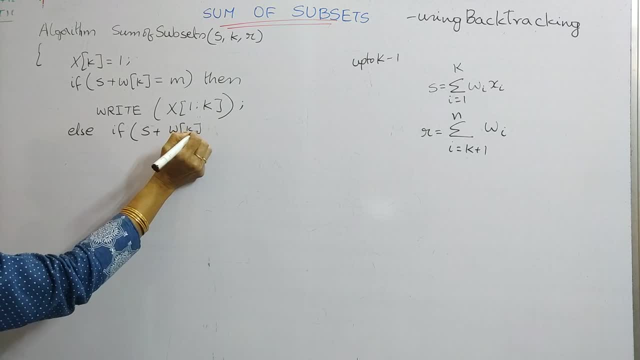 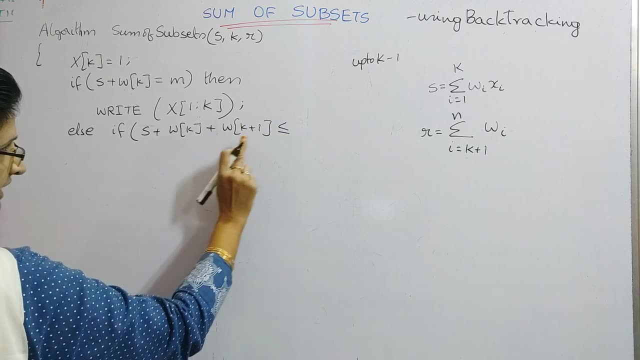 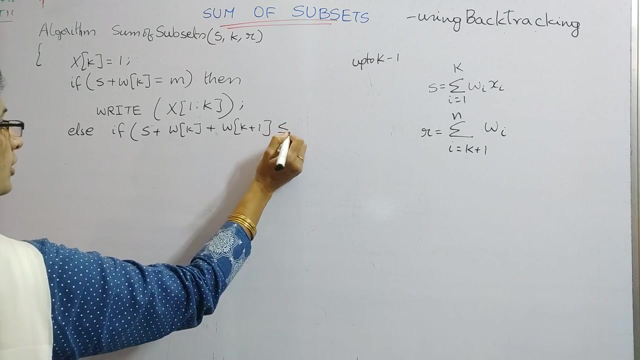 s plus W of k plus W of k plus 1.. So by adding the kth object and the k plus 1th object, Suppose if both, if by adding by both, if it is equal to, if it is less than or equal to. 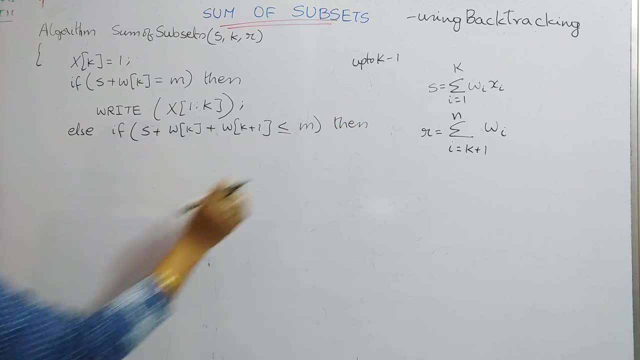 m If it is less than or equal to m Means what? So it is worthable of going in that path. So that means because by adding this object and also the next object, also it is less than or equal to m, And already we have. 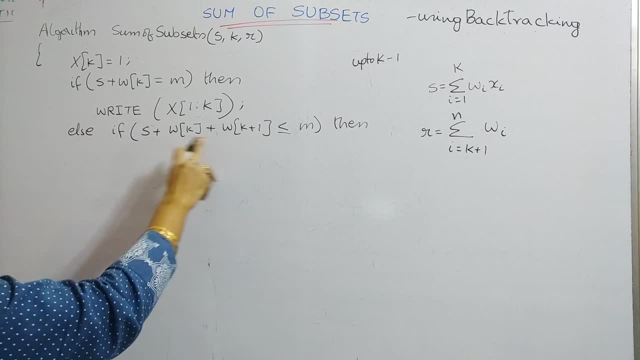 arranged the objects in the non-decreasing order. So that is why, suppose, if this is true, What does it indicate? So you can go in that path. So if you want to go in that path, what you have to do Again, 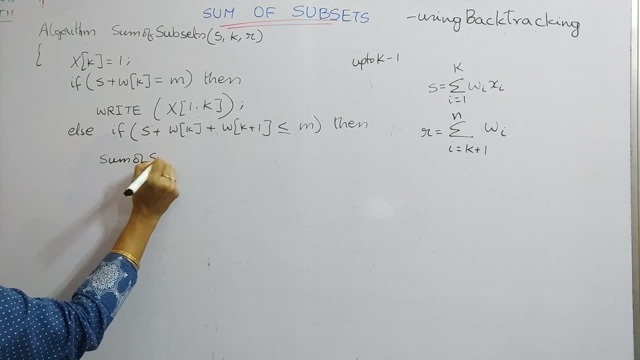 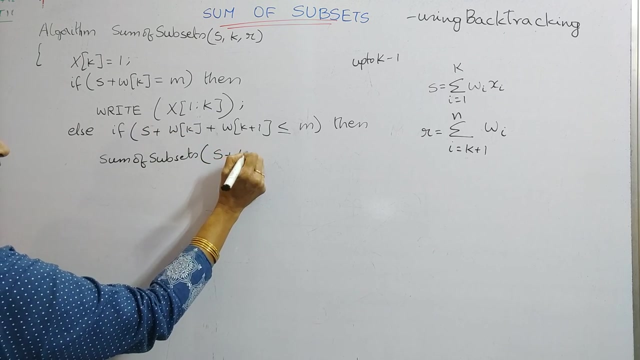 you have to call the same function, that is, sum of subsets for what? So already you have given x of k is equal to 1.. So that means now your x should be added with this w of k. So now for the next call. it should: 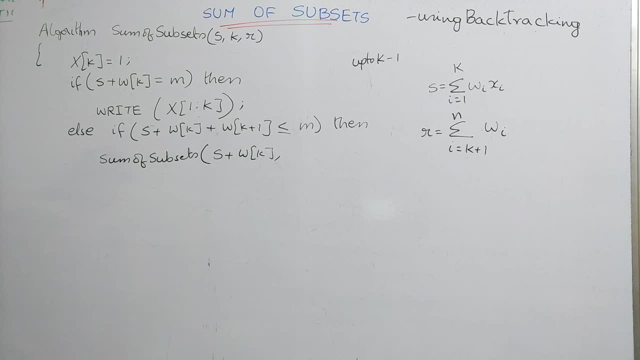 be added, and then you should- you should- pass that parameter. So for s, you are adding the kth object, weight, and you are passing to the next call, and for k, now you have to add 1, that is the next object. So that is why k is equal. 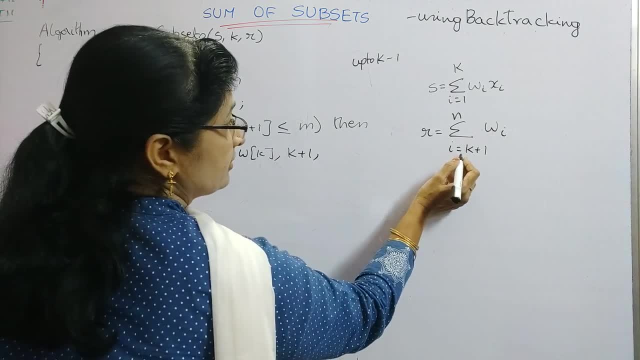 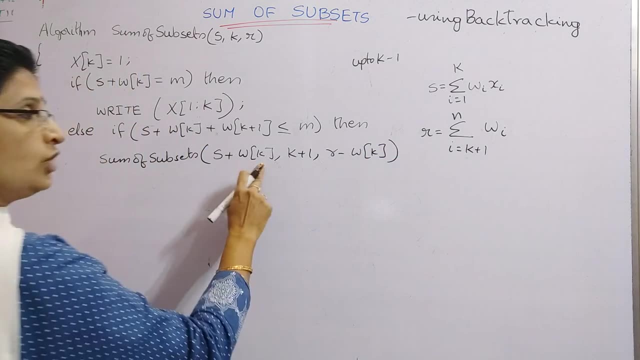 to k plus 1 and for r For r. why we are subtracting the w, w of k? because the decision for the kth object is over. So that means it has been added to this s. So that is why it is removed from. 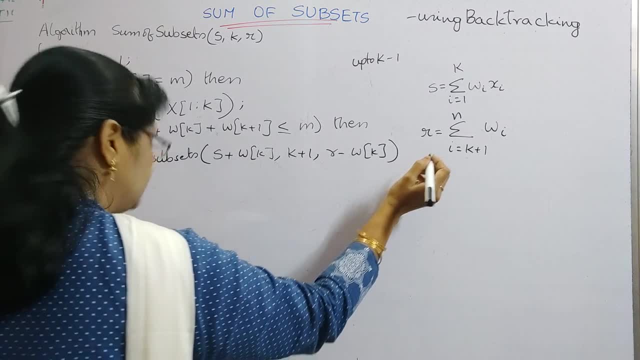 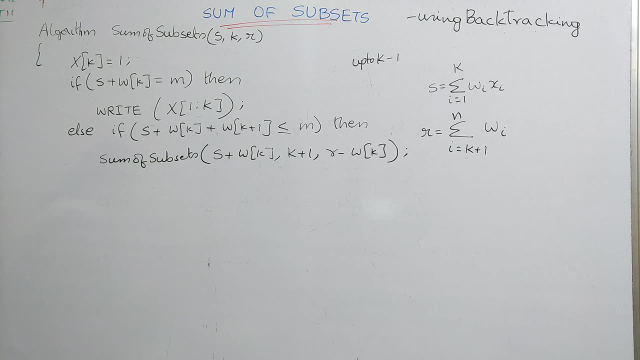 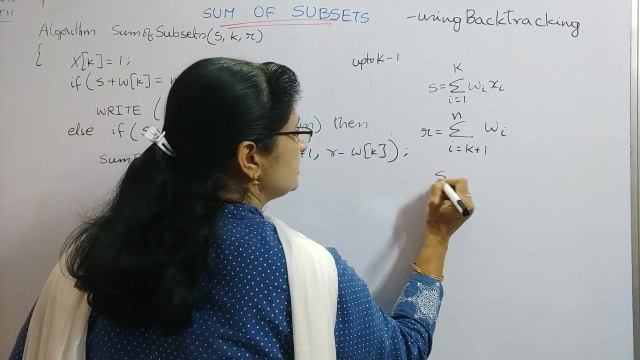 r, It is removed from r. So first, initially, what will be the r? First initially, r will be the total weight of your object. So first initial, for first initial call, for initial call, what will be the s? So till now you have not added any object. 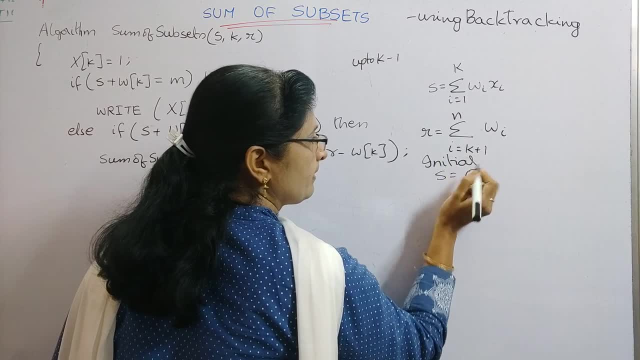 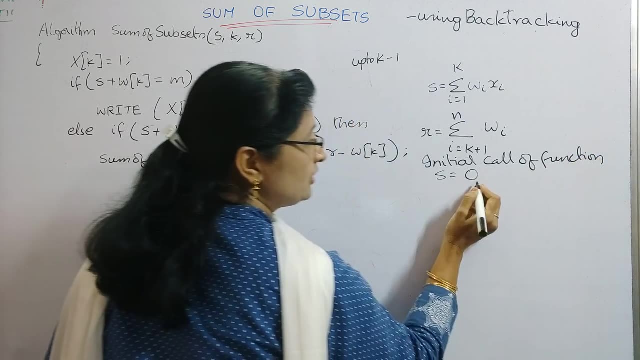 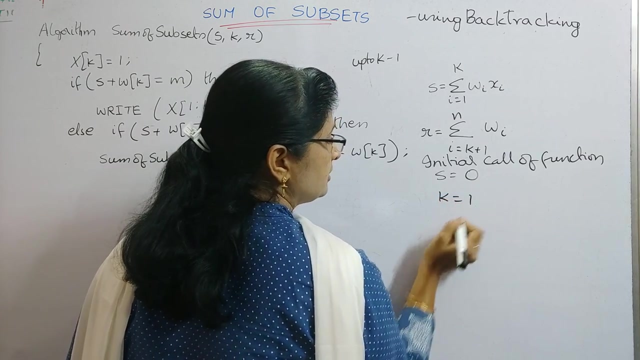 So for initial call, s will be initial call of your function. s will be 0 because you have not added any object. So and k will be 1, and what will be the r? It will be sum of all the objects. 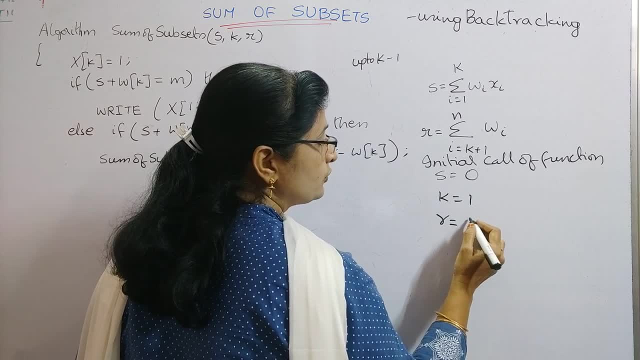 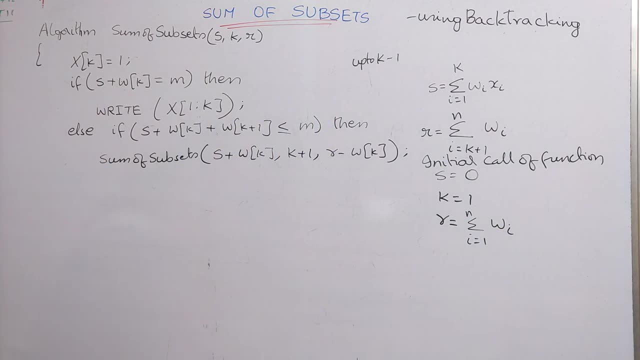 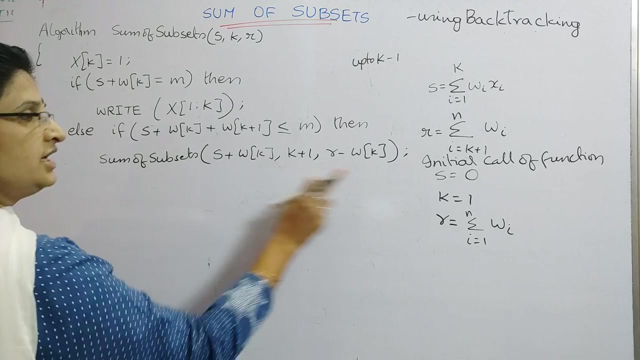 So that is all the objects means it becomes the sum of all the objects. So that is, from i is equal to 1 to n w. So this is how you can give the parameters for your initial call of your function. So now what we are doing in the 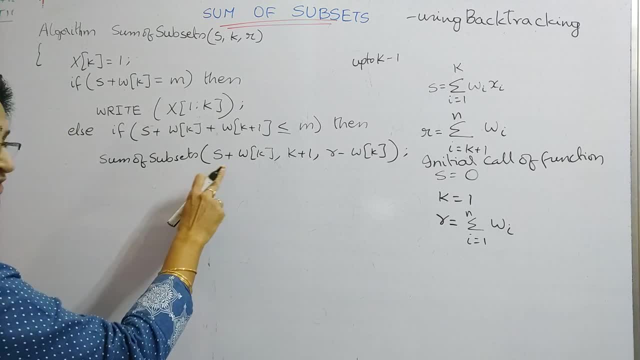 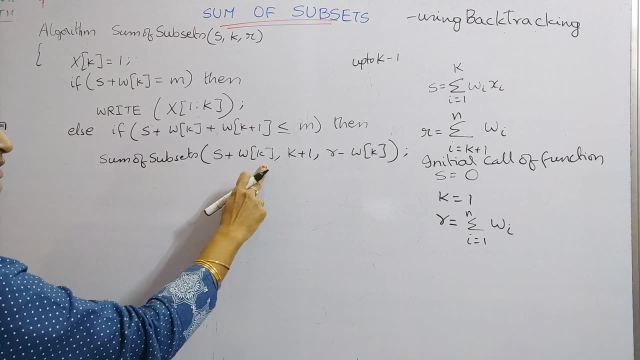 intermediate stage. you are adding the kth object to s and you are subtracting the kth object for r because it has been added and you suppose if it is added means so that means you should give add w of k to s and similarly you should subtract it. 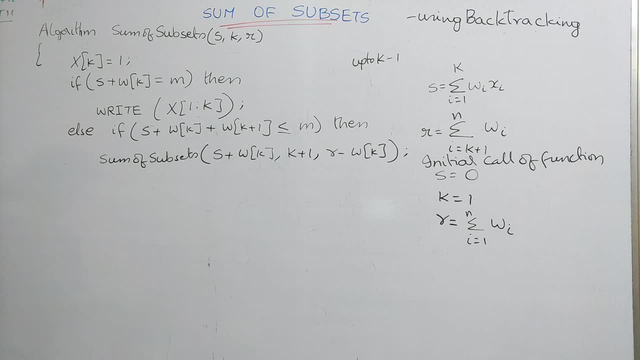 from r. So this is how you can get. that means again, you are calling for the next object. So so next, what we are doing, you are generating, you generate right chain. So that means so this is what x of k is equal to 1 means this: 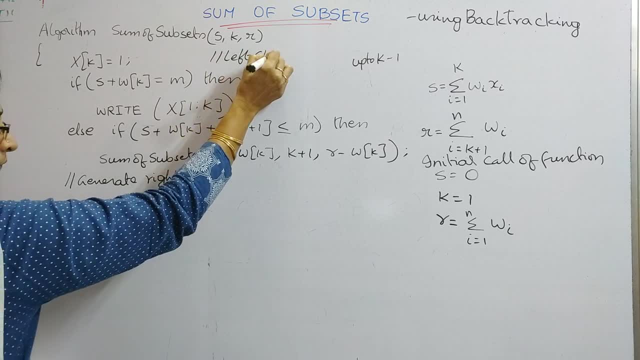 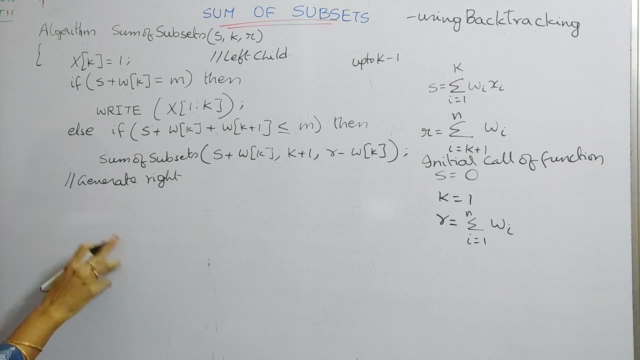 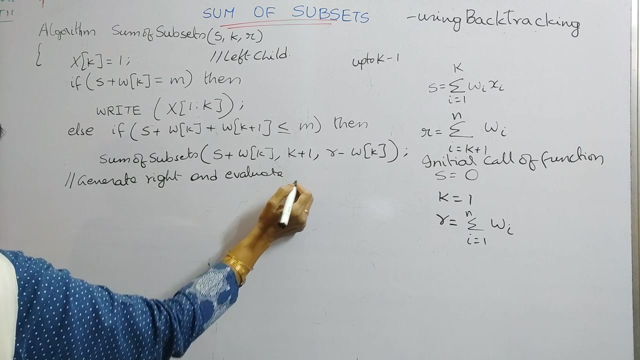 indicates left chain. So similarly for x of k plus The k is equal to 0- also should be generated So that one for that one generate right child and also evaluate And evaluate this, all the parameters, And evaluate all the parameters. 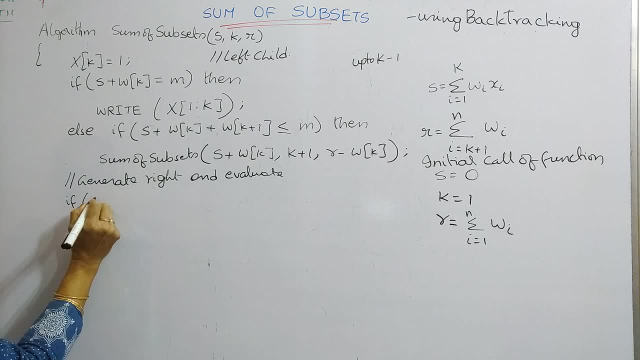 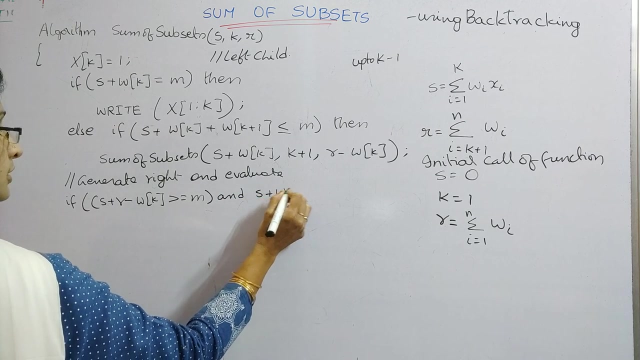 So for that one, what you have to do, You have to check s plus r minus wk is greater than or equal to m. If it is greater than or equal to m and s plus w of k plus 1 is less than or equal to m, 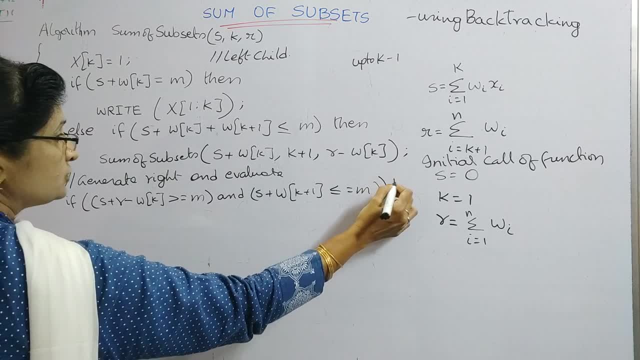 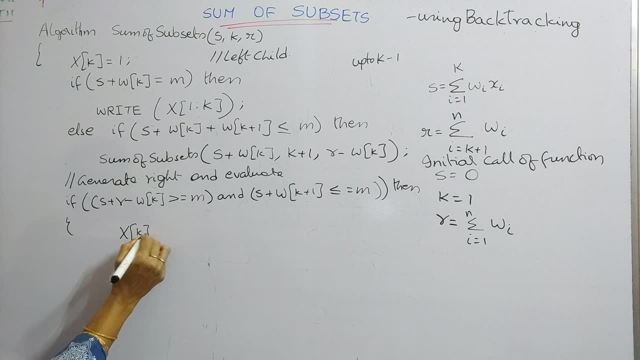 Suppose, if these two conditions are satisfied, then what you will do, You will give x of k is equal to 0. And again you will call the same function that is sum of subsets of s comma k plus 1 comma r minus wk.